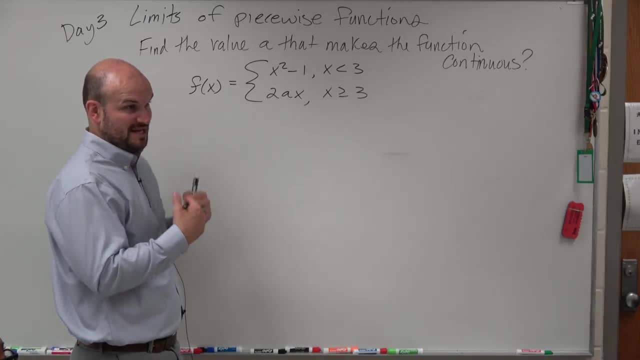 going to be continuous, or we both know it's going to be continuous. that they meet at that point is because we have a continuous function here And then, assuming a is some real number, that's a continuous function, right? So we know that, since we have two, 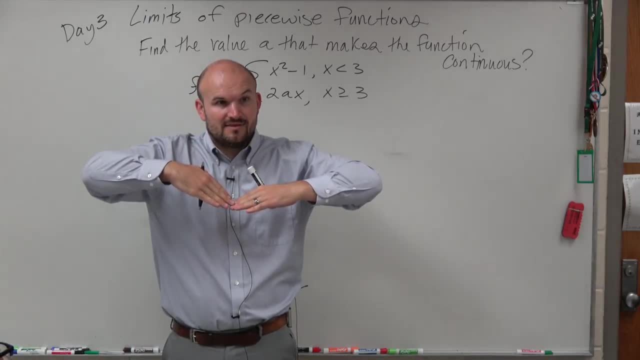 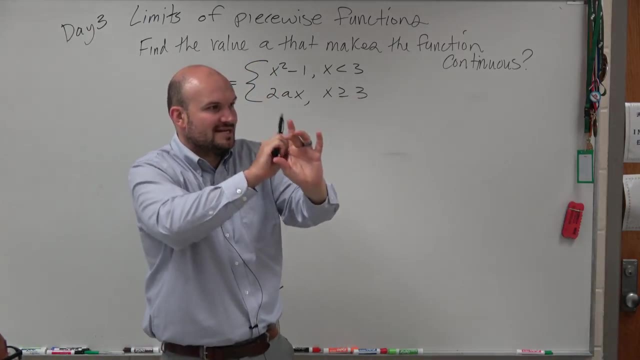 continuous functions. as long as we know they meet, then they're going to be continuous. Does that make sense? Right? And that last piecewise function, the one we did over there, that had a hole, It was obvious. It said: x cannot equal that. 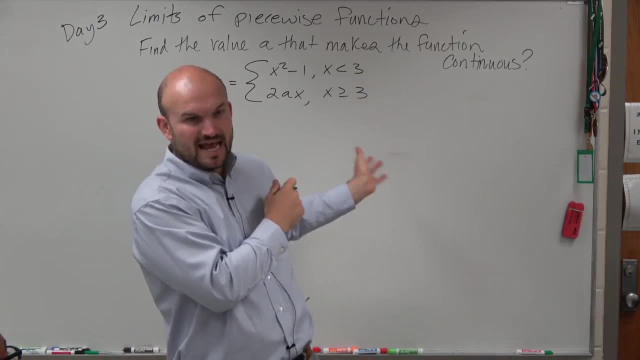 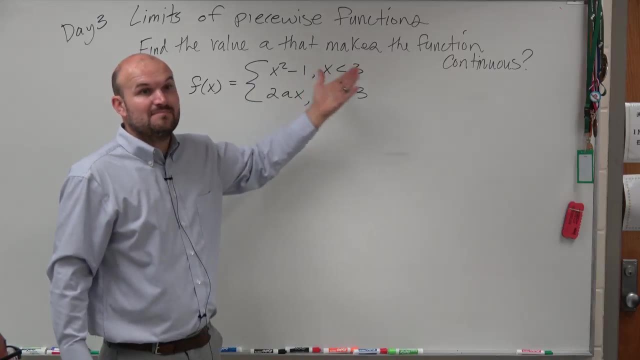 That's a hole, right? We don't have any holes here. Nor do we have any asymptotes, because we're going to talk about those later. So right now we have two continuous functions. We just need to know what values do they meet at? Right. 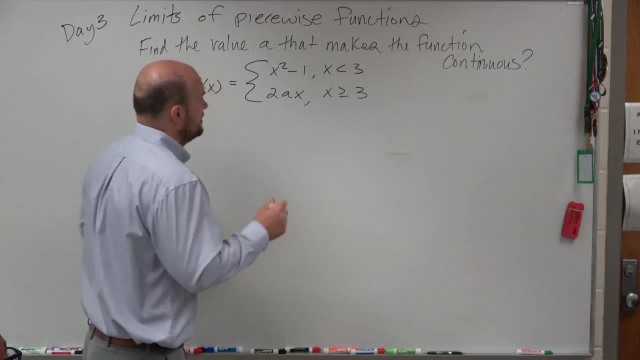 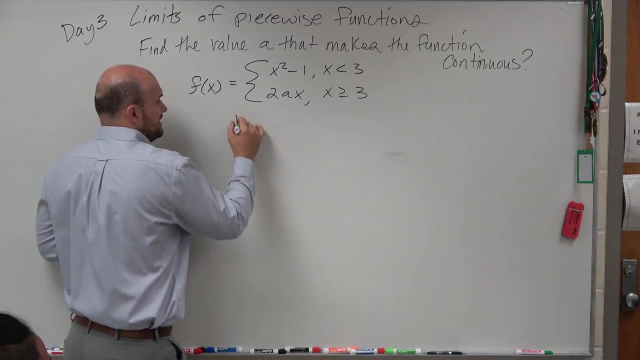 Basically what we're looking at. So what I was trying to refer you guys to is: we know that they're going to meet if their left and right hand limits are equal at 3.. Would you guys agree If I said that the limit as x approaches 3 from the left? 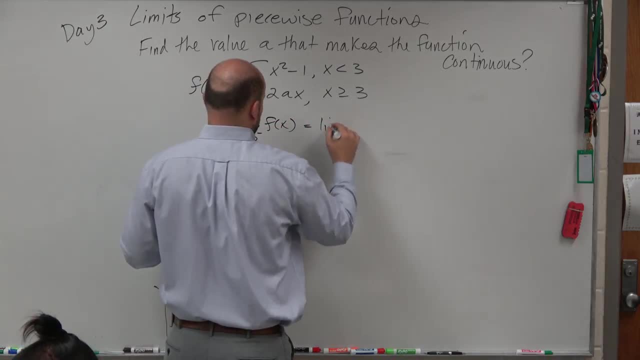 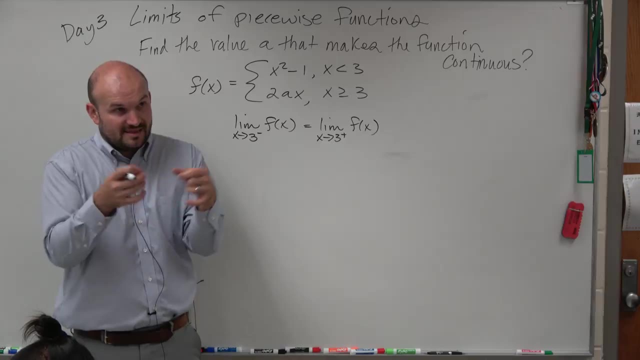 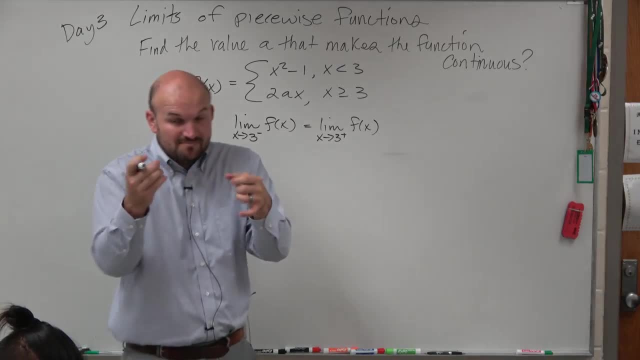 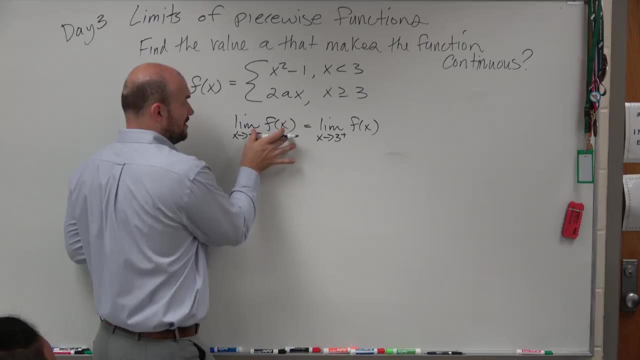 Question from audience. they meet at that point. And if these two continuous functions meet at that point, then it's continuous Right, Correct. So let's see what we have here. We have the limit as x approaches 3 from the left. 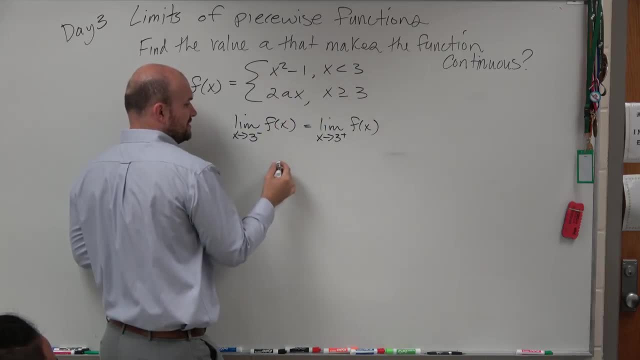 Here's 3.. Here's the function to the left Now again. so here's your x squared. So you have x squared minus 1 has to equal 2ax. But we're evaluating. This is not the left and right limit need to meet. 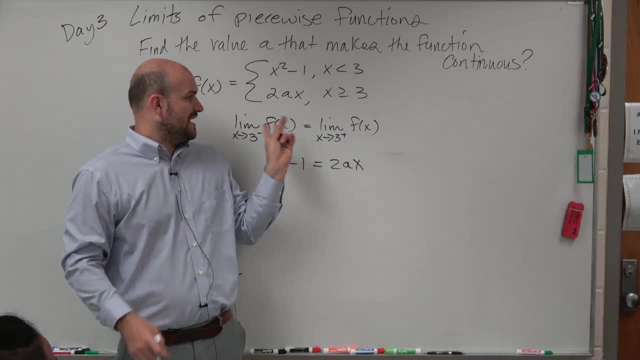 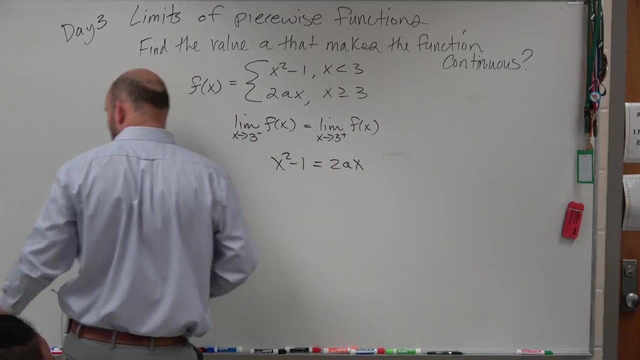 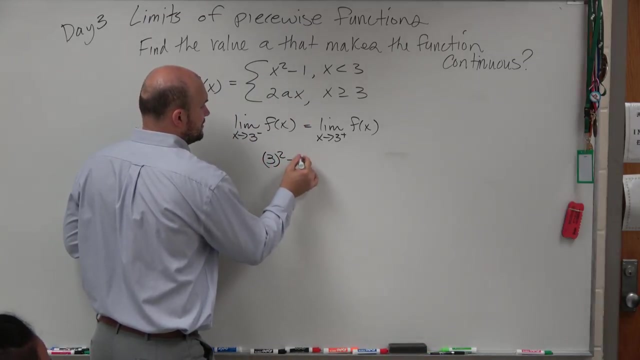 They need to meet at. We want to see what does a need to be if they're going to meet at 3.. So what you'd actually type in, or what you'd plug in, is going to say: what is the value at 3 squared minus 1? 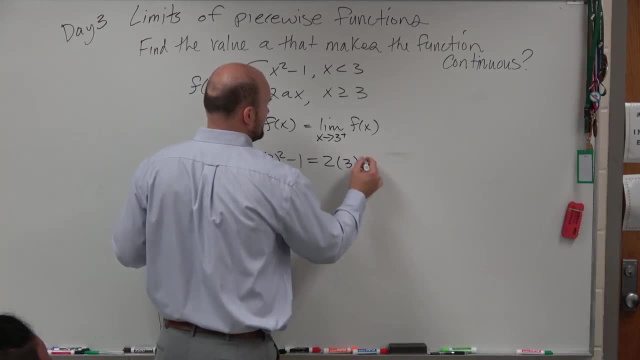 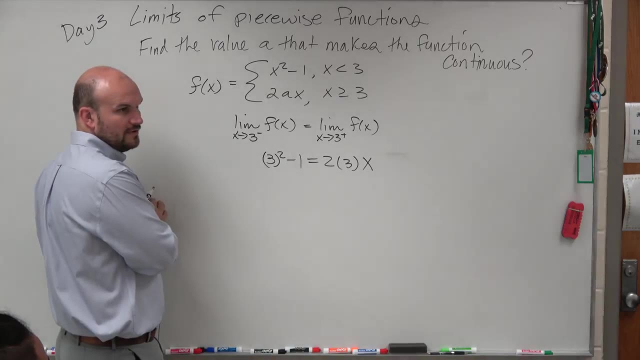 has to equal 2 times, 3 times x. Does everybody kind of see why and where I did that from? You're evaluating the limit left and right hand. side A is trying to find the value that's going to make them meet, But you're evaluating the left and right hand limits of them.